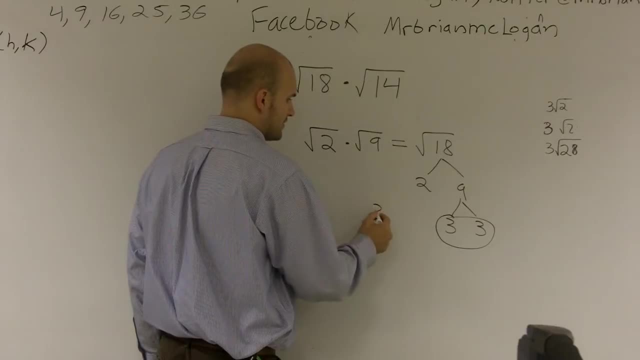 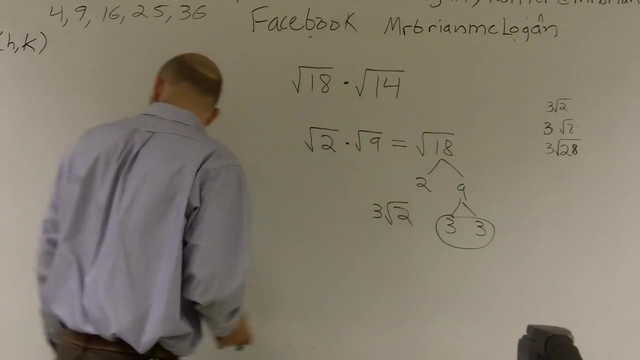 I'll have three. it comes out times the square root of two. since that's left over, I can't take the root that out. So that's what would happen if you can just multiply this, so you could multiply 18 times 14. I don't know. 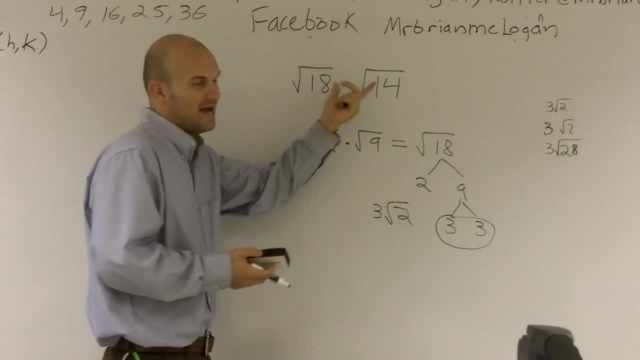 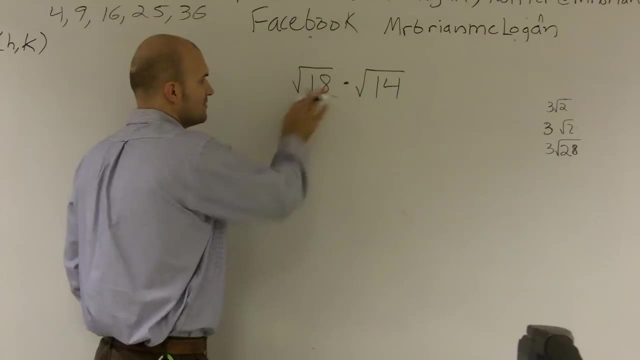 what it is off the top of my head, but I don't really want to try to turn, turn that and then try to factor that out. that seems like too much work for me. so another way that we can do this and another way to factor our- I'm sorry to simplify your radical is: I'm going to look at simplifying both of these first. 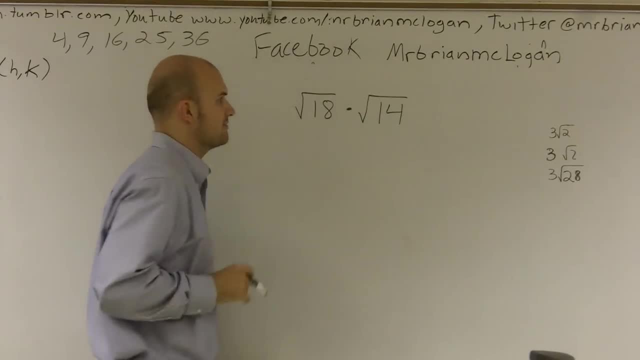 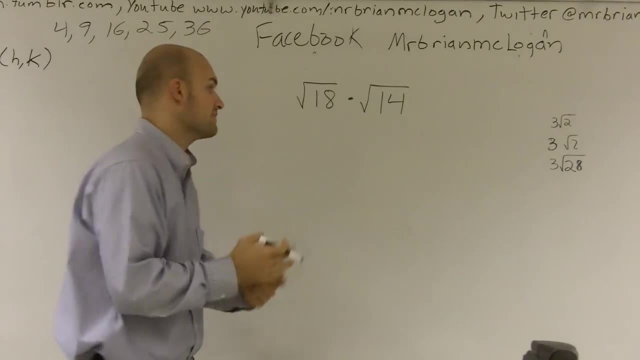 and then multiplying them. so another way you can simplify radical 18 is I can say: what is a square number? remember, square numbers are four: 9, 16, 25.. What square number evenly divides into 18?? And I figure out that 9 evenly goes into there two times. 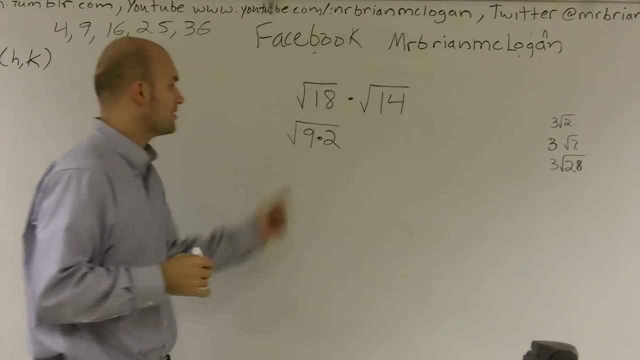 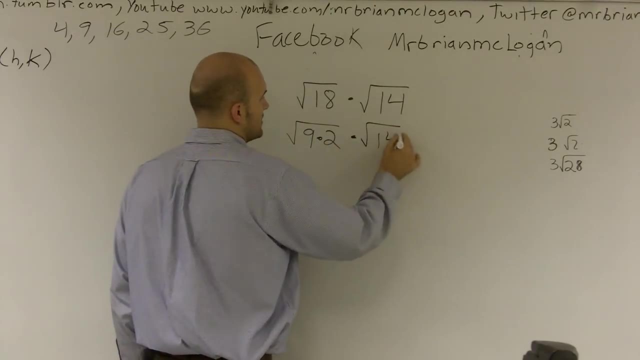 So I'm going to rewrite 18 as a product of a square number times another number. So I can rewrite 18 as square root of 9 times 2 times square root of 14.. Well, the reason why this is helpful is because the products 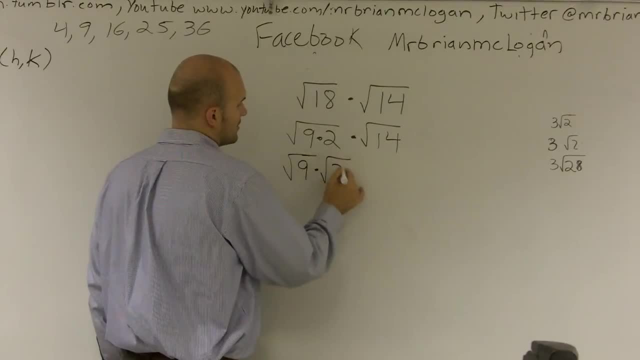 or the rules of radicals, allows me to split up my two radicals. So since I'm doing multiplication, I can actually split up taking the root of both of these. Therefore, now I obtain 3 times square root of 2 times square root of 14.. 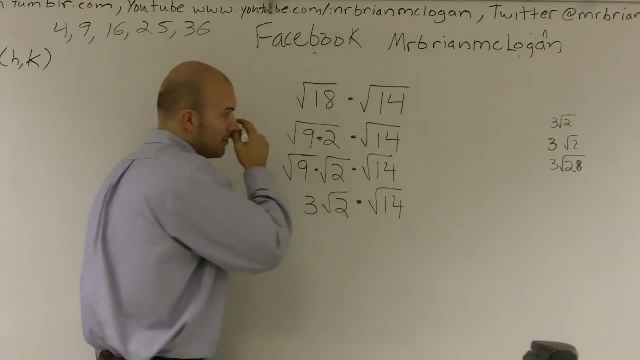 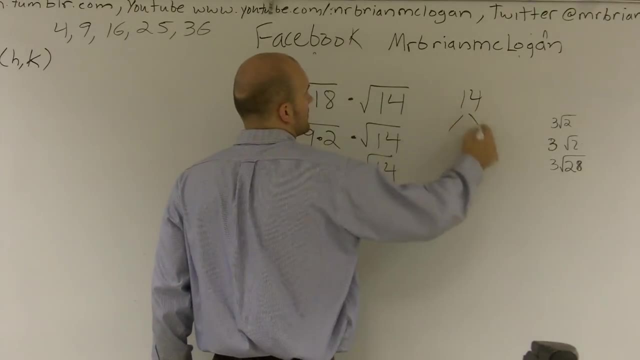 Now I haven't done anything with square root of 14 because I intrinsically already know that you can't reduce the square root of 14.. There is no number If you're going to factor this: 2,, 7,. 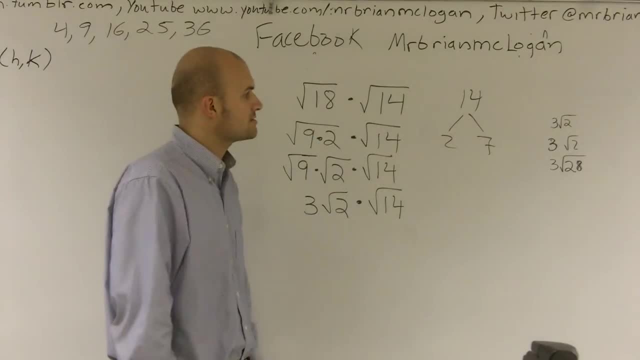 those are both prime numbers, as is 14 is a prime number as well or not a prime number. But 2 and 7 are both prime numbers, So therefore there's nothing else. you can factor that for. So now I have 3 times radical, 2 times radical 14.. 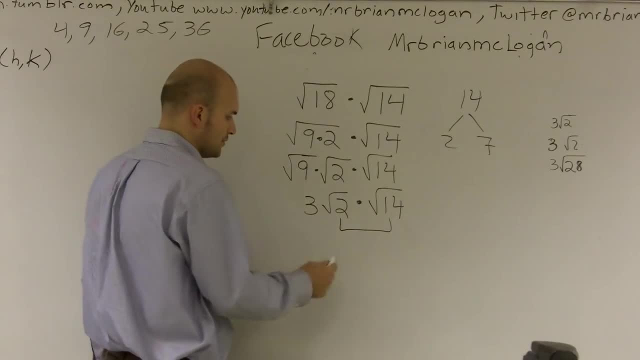 Well, I can multiply these two, since I'm taking the radical of both of them. So I have 3 times. the square root of 2 times 14 is 28.. And then again, last check, I go and see: is there any square number that divides evenly into those?